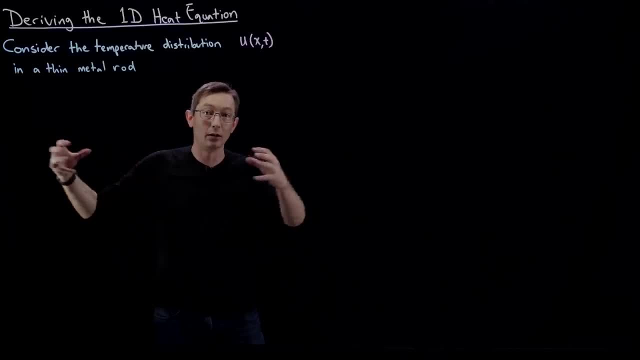 physics in general is that we kind of keep track of all of the you know some quantity like thermal energy and we derive a conservation law-based PDE for that. So I'm going to jump right in. I'm super excited. This is one of my kind of favorites, Okay, so we're going to consider. 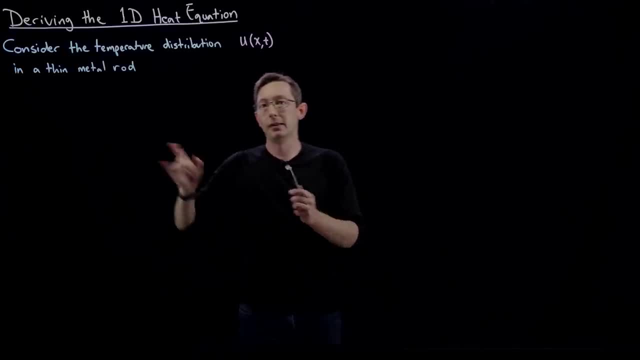 the temperature distribution u of x and t in a thin metal rod. So let's actually draw like a little you know. you can just kind of imagine this is a wire or a little piece of you know metal that you can pick up at the hardware store. And u of x and t is the temperature. 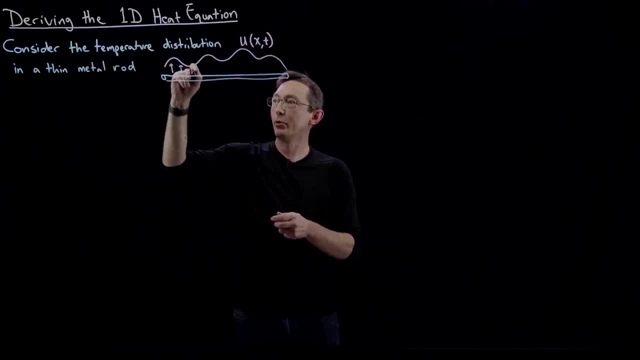 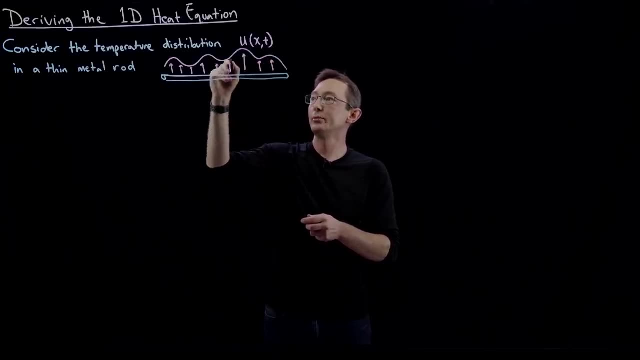 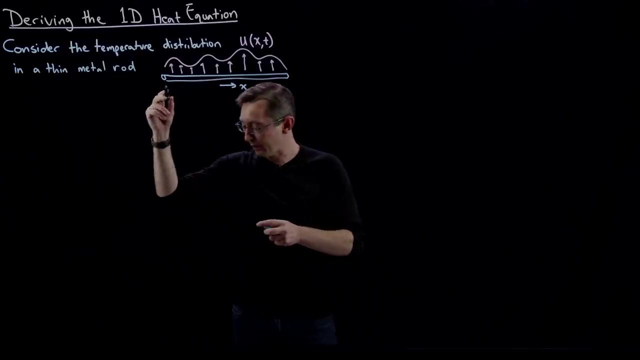 distribution, literally the temperature at every point in x. So x is how far I am along this thin metal rod. U is the temperature distribution and it's evolving in time. Okay, so let's just draw x, And the boundary conditions are going to be zero and l. x equals zero and x equals l And u of. 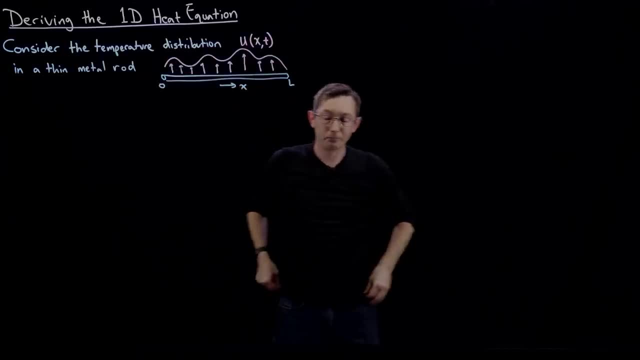 x and t is this temperature distribution that's changing in space and in time, And so what we're going to do is we're going to use common sense that there's like a conservation of thermal energy in this thin metal rod, And we're going to keep this apart and we're using Sharknado to know like the distribution that 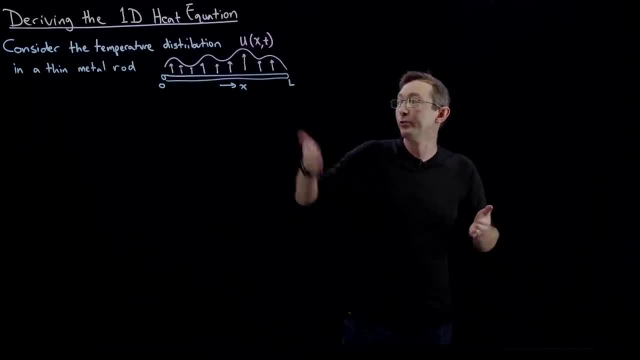 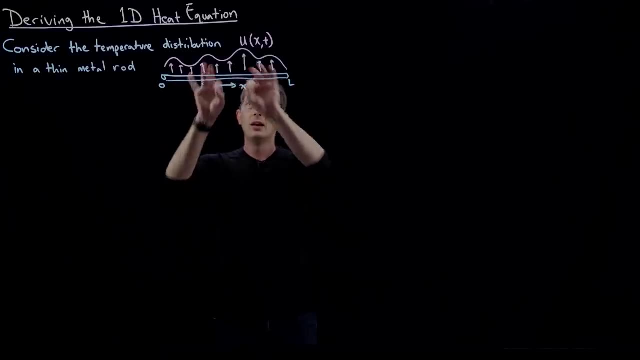 Ah ن n s x oui derive a partial differential equation. that has to be true for that conservation to be satisfied. now i'm going to assume a couple of things here. i'm going to assume, for example, that this is an: 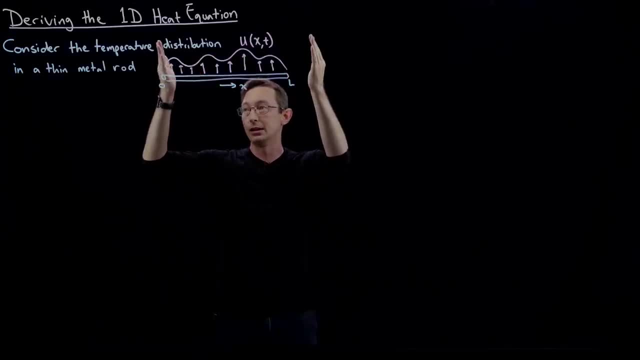 insulated rod. so we're going to put kind of a styrofoam sheath around it and maybe i will, you know, fix the temperature at the boundary conditions or insulate the boundary conditions. and i'll start with some initial temperature distribution u of x at time zero. so that would 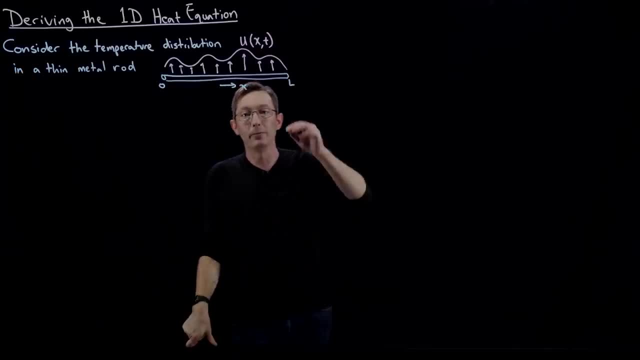 be my initial condition and what we eventually want to do is: you know, we're going to derive that partial differential equation, but then we want to solve that pde for the distribution u of x and t everywhere in space. at later times- t- i want to know what the temperature distribution will be. 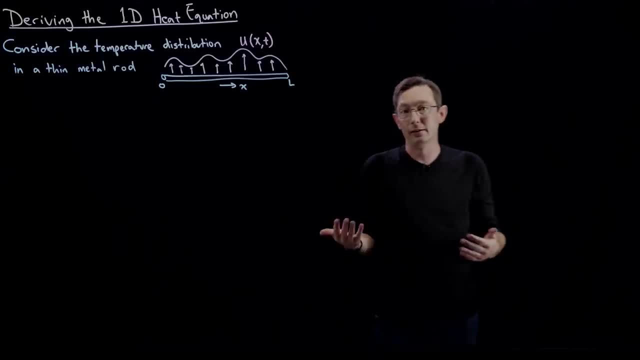 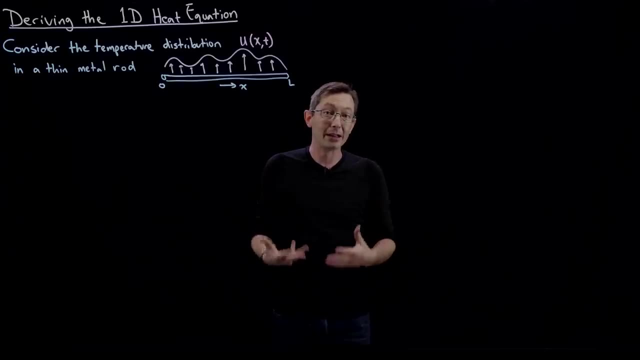 like in the future- and this is important for lots of applications. right predicting the thermal distribution in an object is a critical capability. when we design engineering systems like a space shuttle re-entering the earth's atmosphere, we better be able to tell how the temperature distribution on the surface. 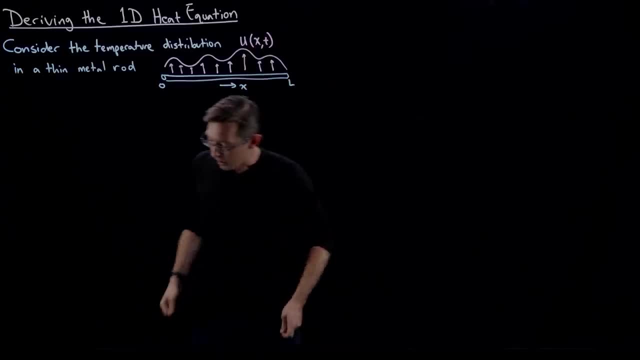 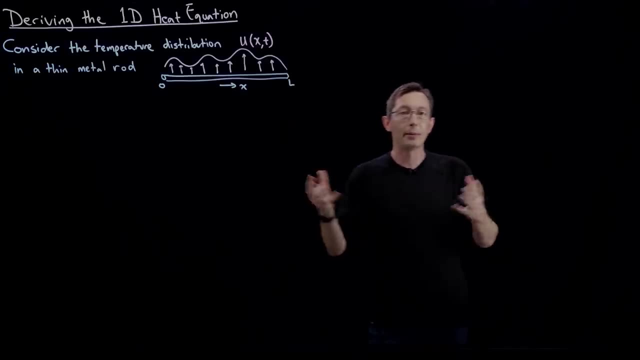 changes in space and in time. okay, uh, good, so let's jump in. um, we are, yeah, essentially going to, like i said, use common sense, uh, to derive this partial differential equation. so let's start doing this, and i want to write this out in words for first. so the rate of change of heat energy in time. 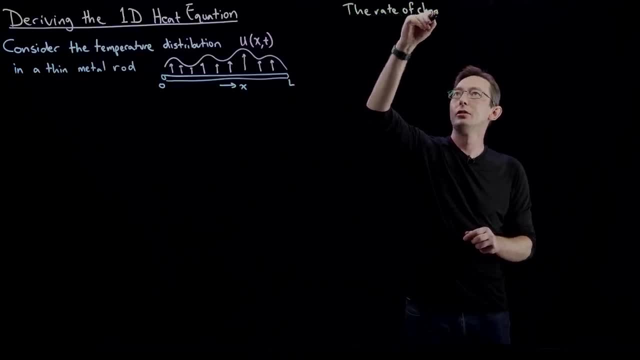 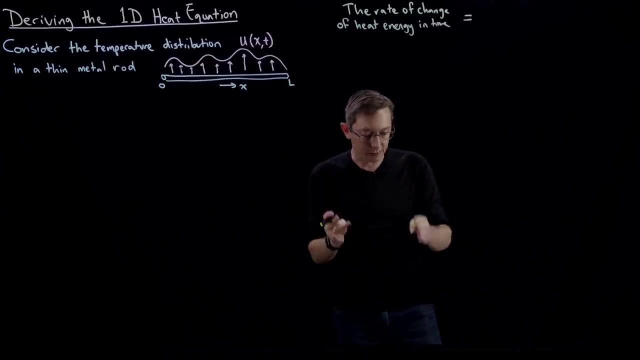 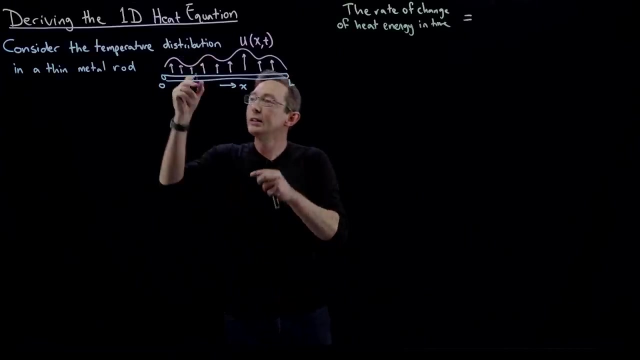 is the rate of change of heat energy in time is going to equal, is going to equal the heat flux through the boundary at every point in space. if i take this is actually going to be a really important thing. we're going to take a little segment of this and we're going to zoom in with the laurier and we're going to zoom. 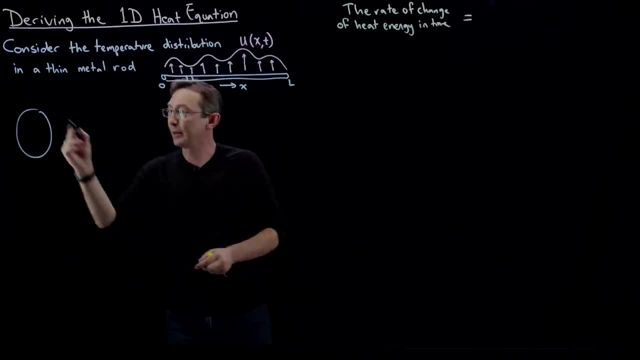 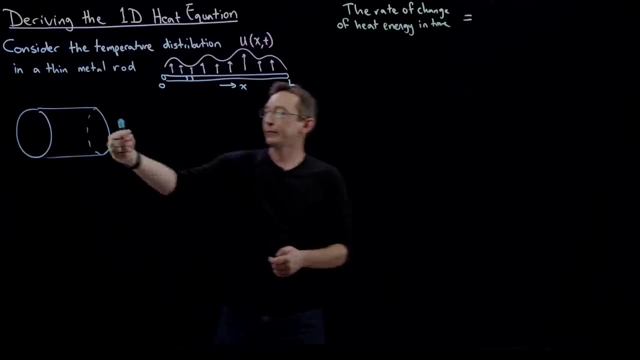 into that segment. we're going to zoom in to a little segment here. okay, if we zoom into that little segment, then there will be heat flux through the boundary into the next element and if it's insulated it won't go out to space, but it'll only go to its neighboring little elements. 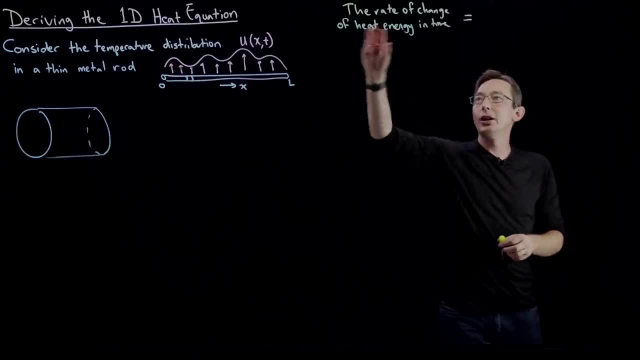 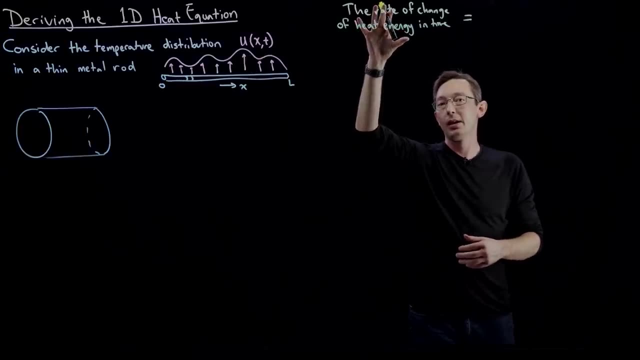 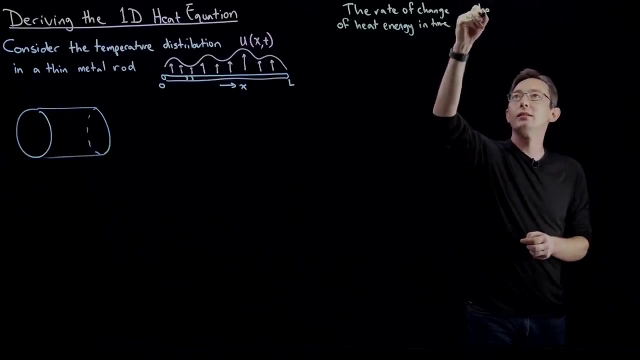 to the left or to the right of it. so the rate of change of heat energy in this, uh, this rod at in time is going to equal. the only way it can change is if heat energy fluxes out through conduction to its neighbors. so heat flux, heat flux through the boundary, through the boundary. 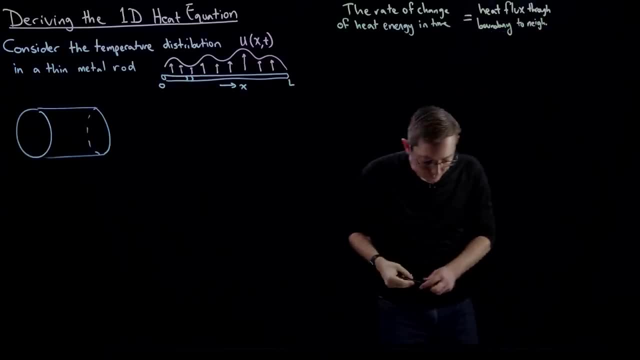 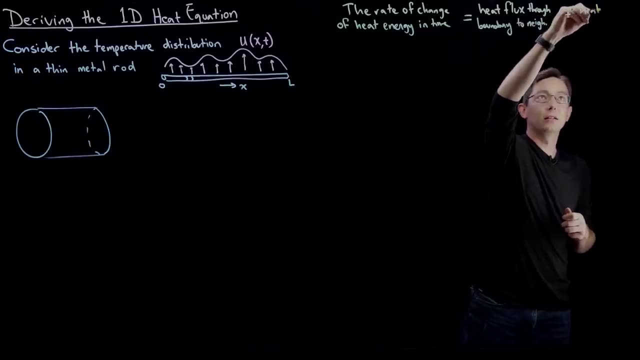 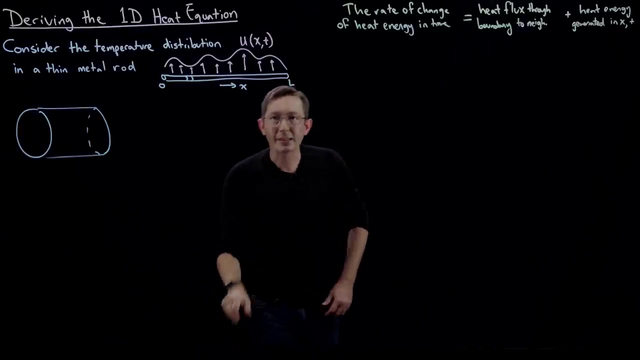 to its neighbors, plus any heat generated at a point in space, plus any uh heat generated, heat energy generated energy generated in kind of x and t and at any point in space or in time. and so, for example, maybe i have a fancy way of heating up a little local patch of this and putting in heat energy. maybe i can inject. 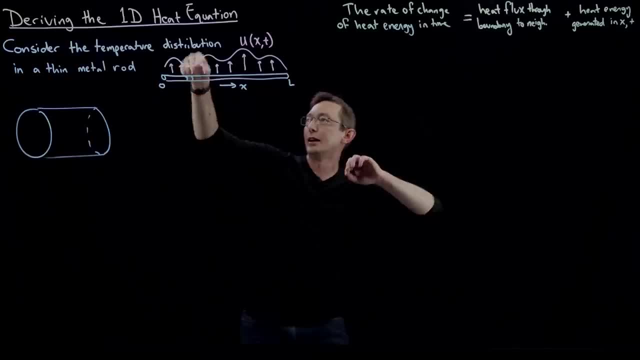 heat energy with a blow torch at this point and create, you know, this kind of heat spike here. that would be, uh, as you can see, i'm adding heat energy like this. or maybe my thin metal rod is not actually made of, you know, uh, copper or something like that. maybe it's made of plutonium and it's actually generating. 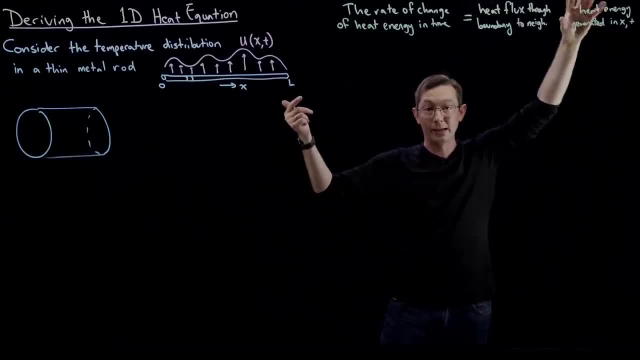 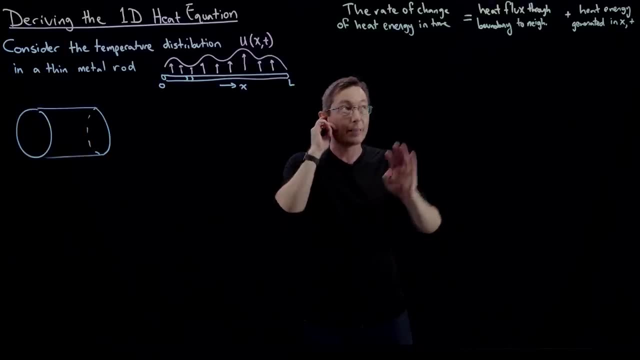 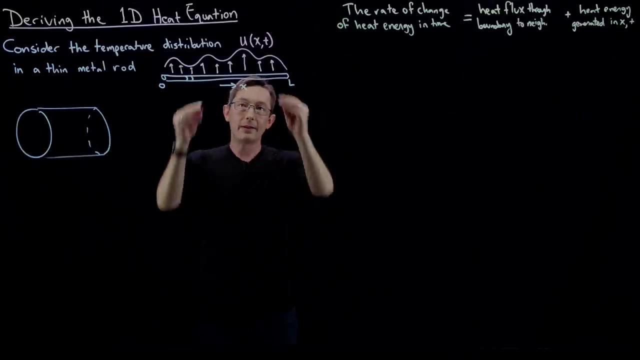 you know, heat, radiate, heat through some atomic process. maybe there's some, uh, some atomic process generating heat energy at each of these local segments. now, the cool thing about this is that this basic- uh, this is just a basic statement. uh, this is just a very, very general statement that we can use to explain the way that the 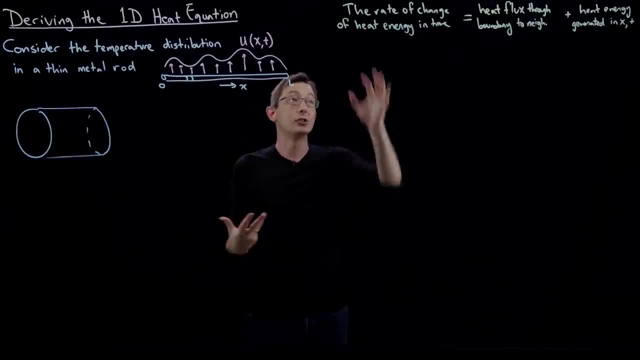 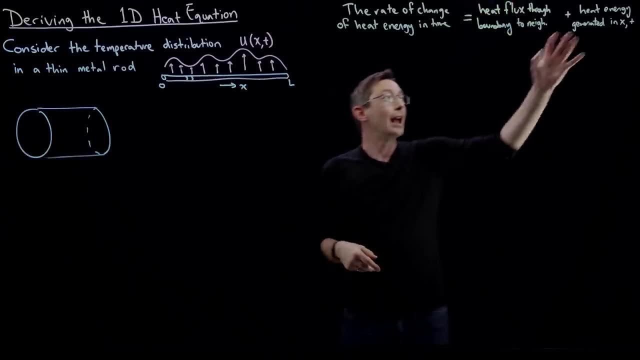 total heat energy. the total thermal energy of the system can change in time, is through heat flux through the boundaries or, if i zoom into a little patch, through its neighbors, and if there is heat energy generated at each of these local pieces in time, either through you know. 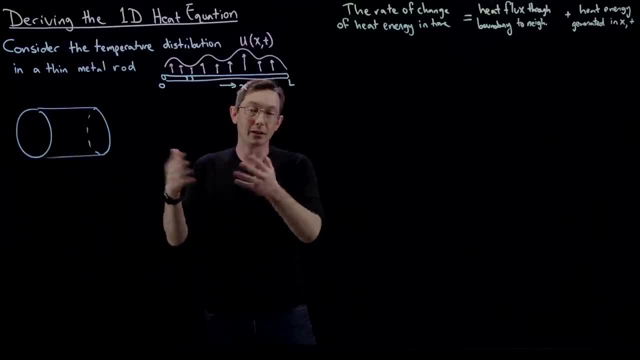 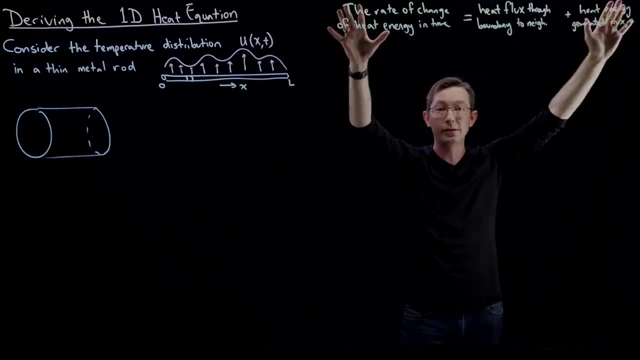 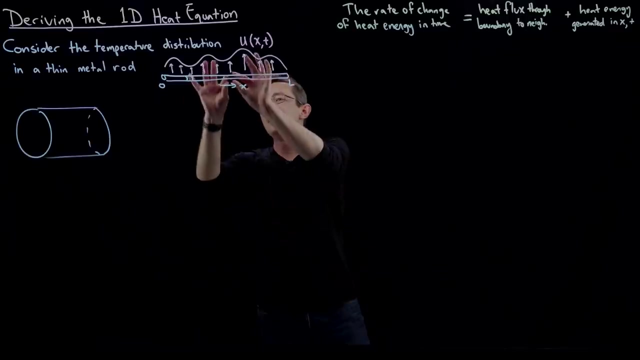 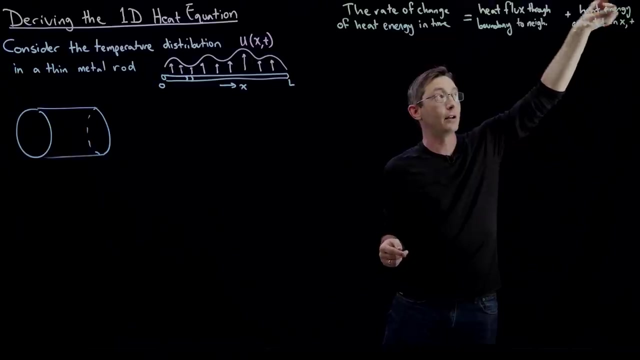 external forcing or through, you know, molecular atomic processes like, like fission, and so this is just a very, very general statement of the conservation of thermal energy. this is basically always true, even for exotic materials. this is going to be true. even if my boundary was not insulated, then i could have heat energy lost through radiation. this would be. i would be able. 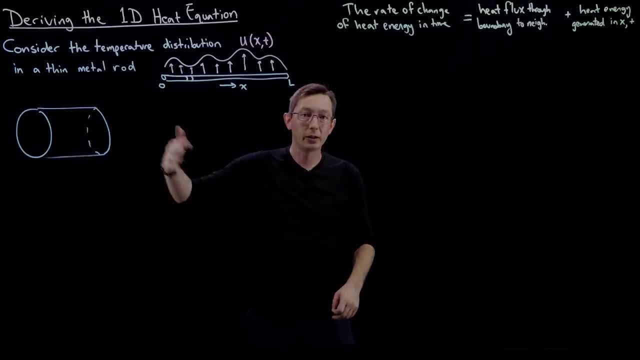 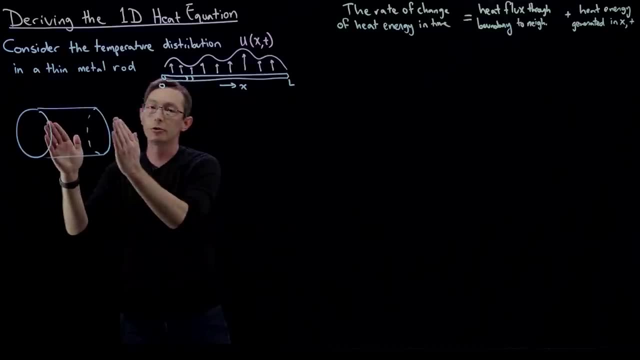 to include radiation effects in here as well: thermal effects, nuclear effects, radiation effects- and it's true integrated over the entire domain, but it's also true when i zoom into a teeny tiny little, uh, local segment of the domain, and that's going to be a really important point. 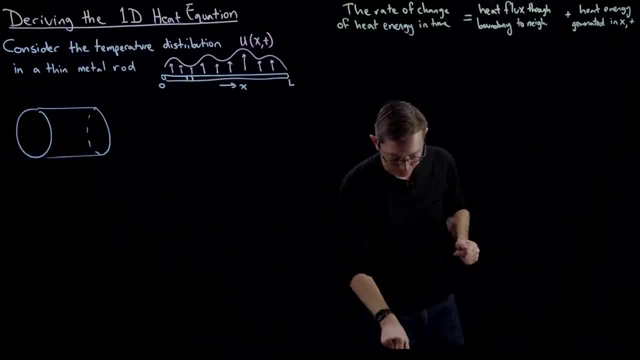 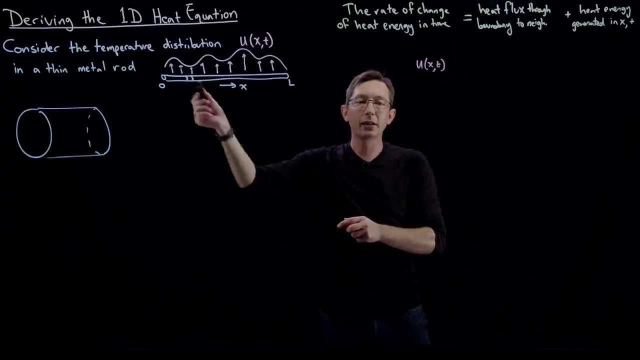 so now i'm going to write each of these three terms in math, okay, and maybe i will do this in pink here. so the total heat energy is given by our temperature, u of x and t, but the a particular material- let's say this is copper or lead or whatever material this is- has some physical 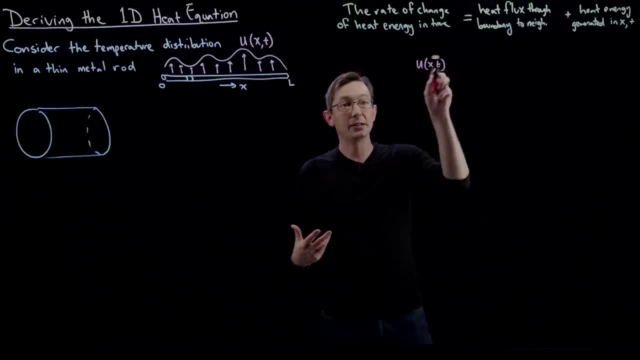 properties that tell me how much heat energy there is at a given temperature and at a given, you know, mass or density. so it's not just u of x and t. i have to multiply this by rho of x, the density, and by c of x, the specific heat. so i'm going to write these down otherwise. 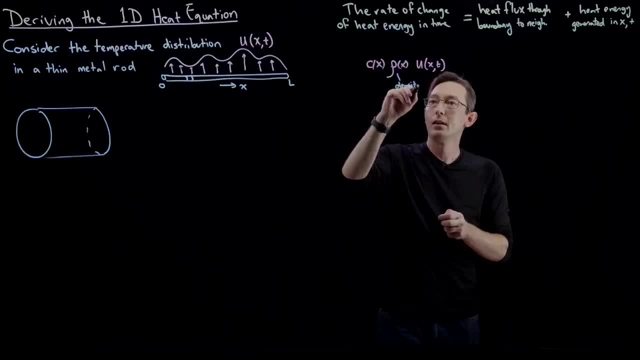 i'll forget. so this is the density, this is the specific heat kind of the. you know the heat capacity of the, of the overall temperature. i'm going to write this down in simple object. and this whole thing here is the heat energy. The heat energy in some. 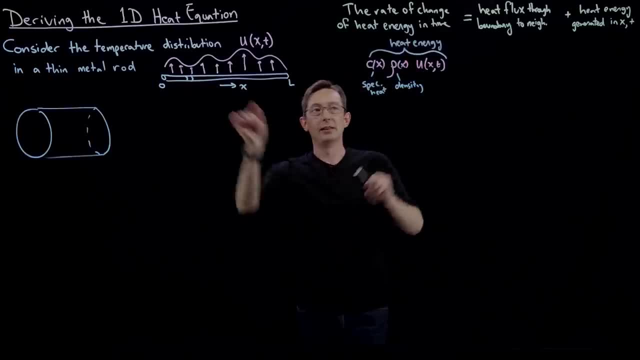 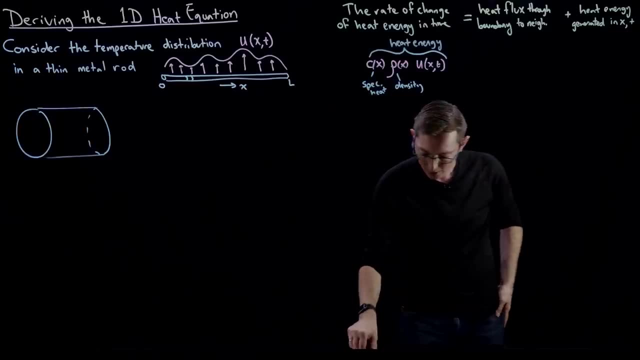 little kind of infinitesimal segment of this. this would be the heat energy in that little infinitesimal segment. You can multiply this by a delta X if you really want. okay, And what we're saying is that the time rate of change of this. 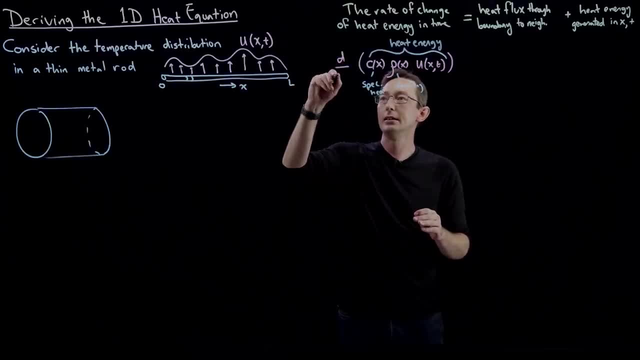 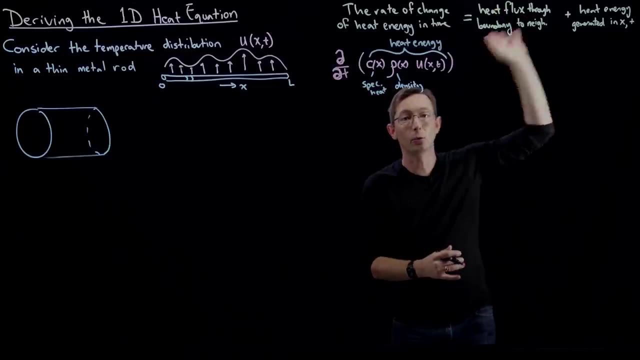 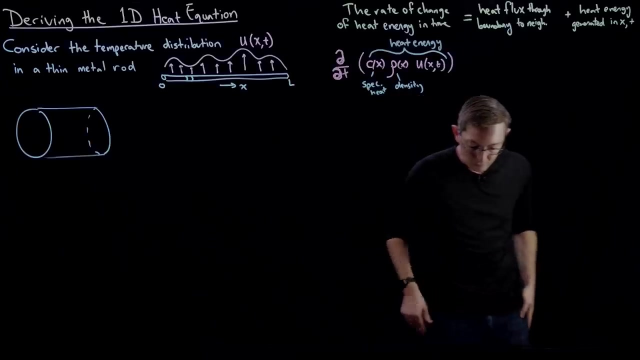 the DDT of this quantity. DDT, really, this is a partial derivative with respect to time. partial DDT of the heat energy can only, there can only be a change in heat energy due to flux through the boundaries or source or sink terms, heat energy generated or lost at points, at points in space. Good okay. 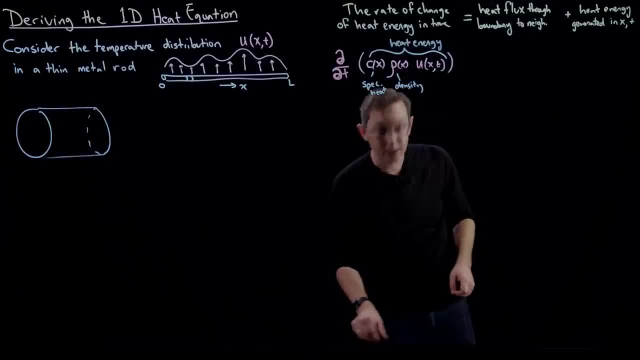 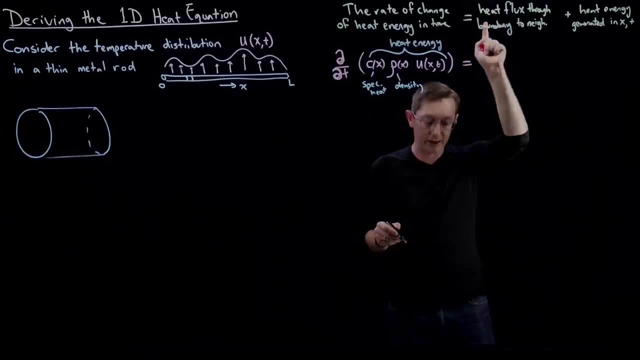 And so this is going to equal. so let's keep the color scheme here. this is going to equal heat flux through the boundary at each point in time, and so this is going to equal, so let's keep the color scheme here. this is going to equal heat flux through the boundary at each. 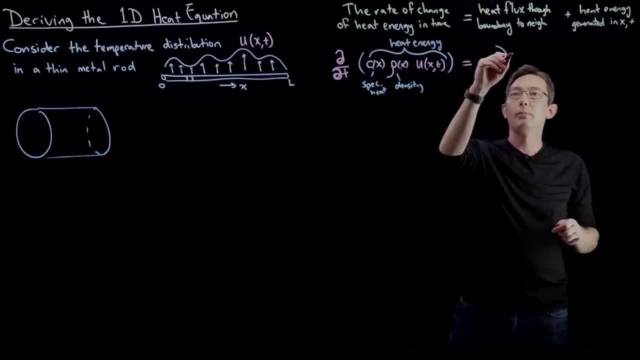 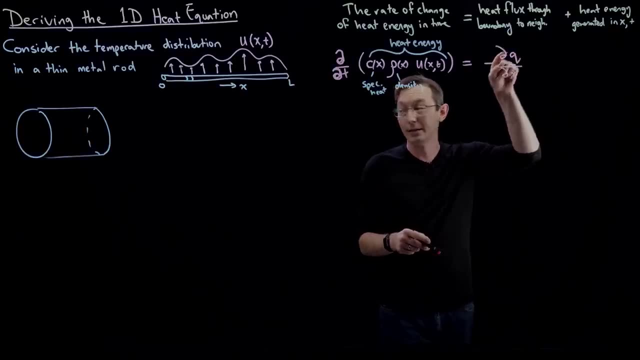 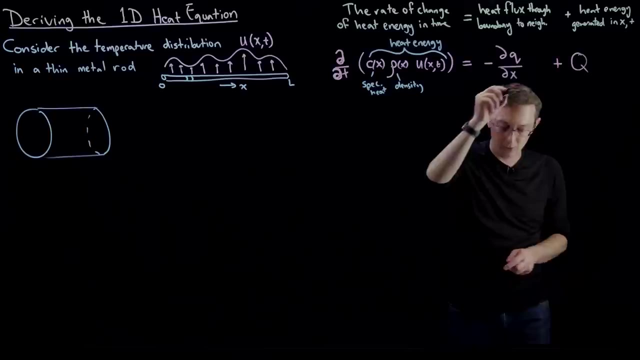 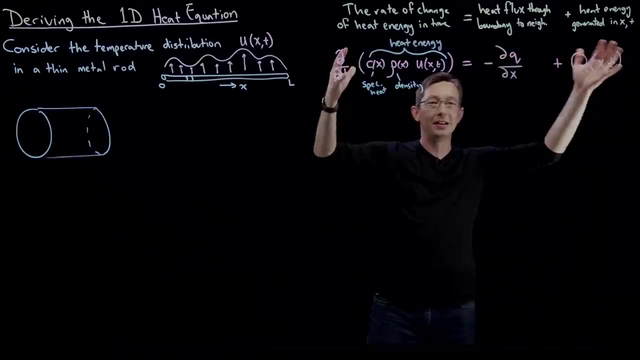 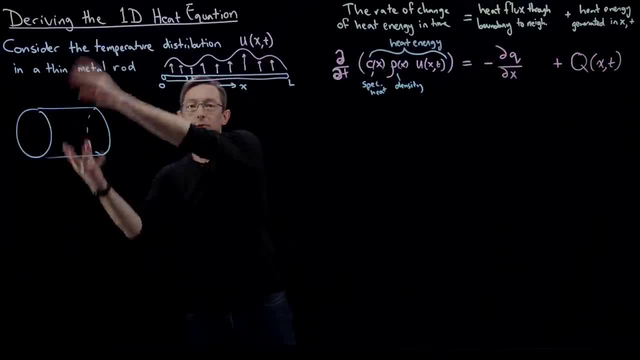 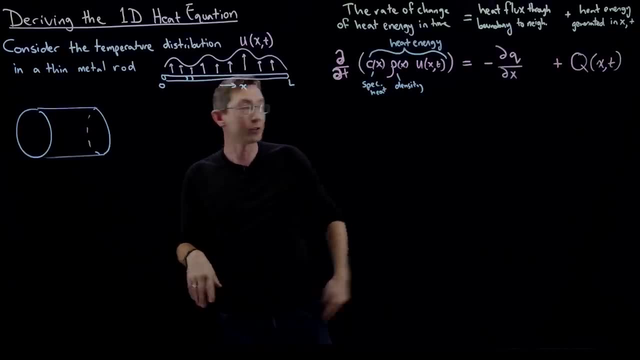 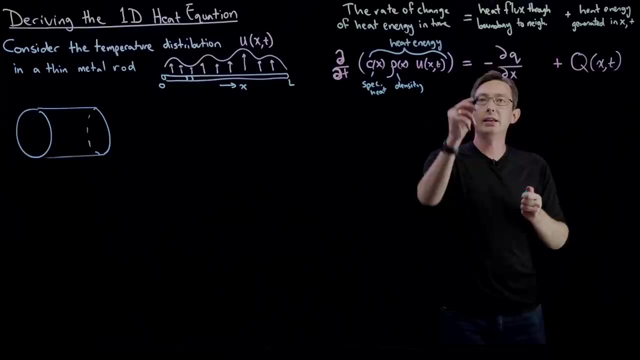 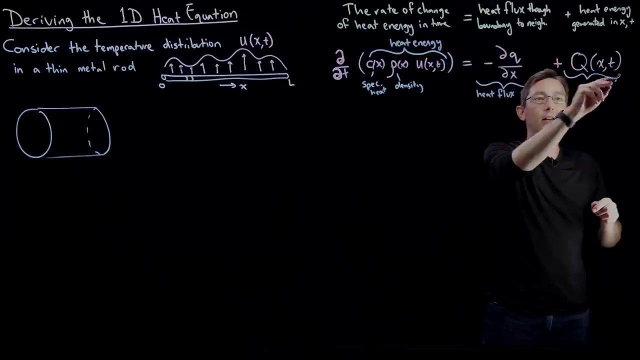 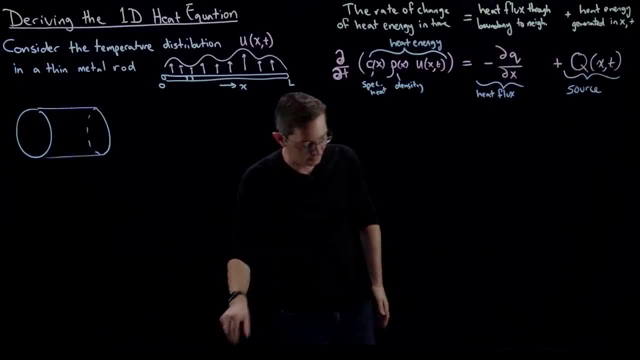 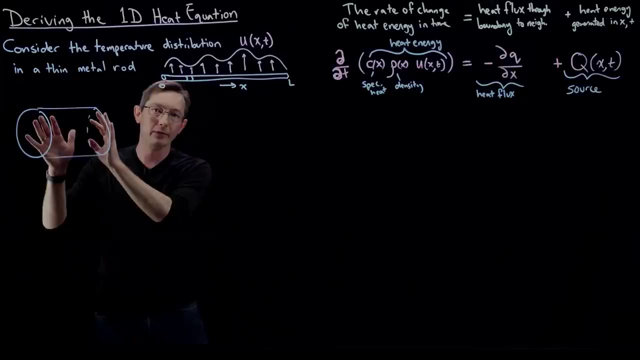 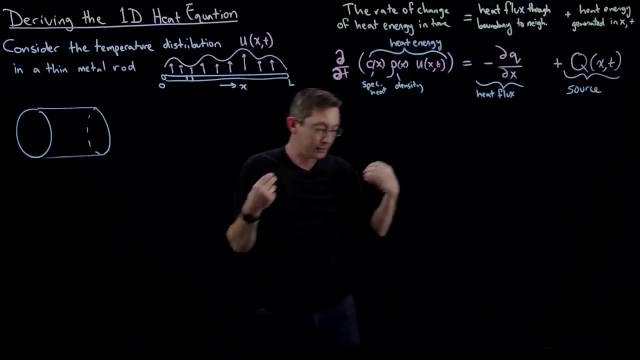 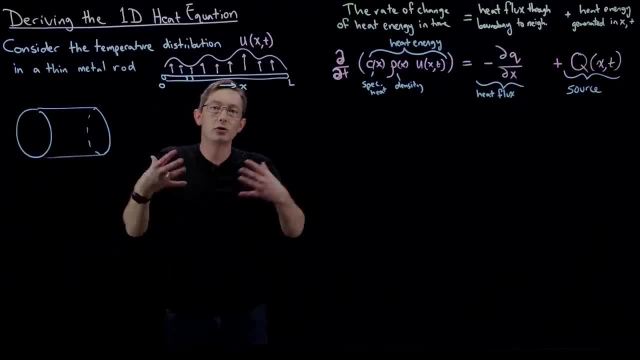 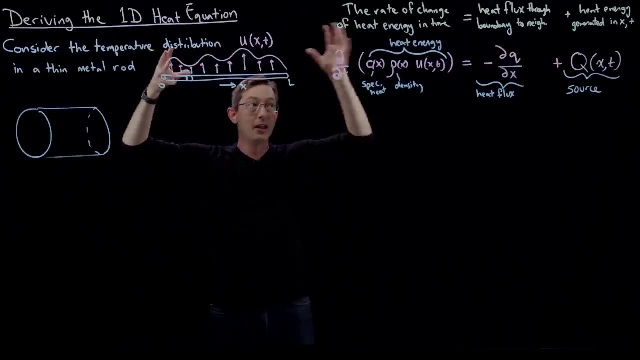 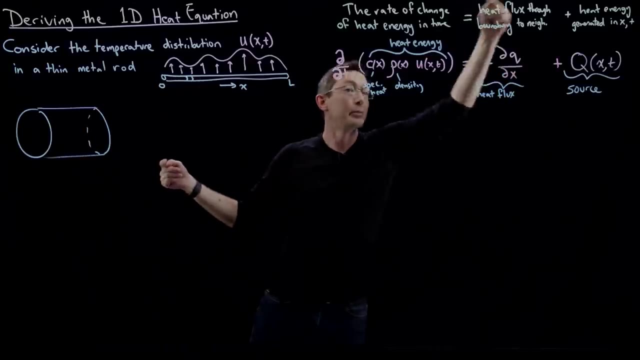 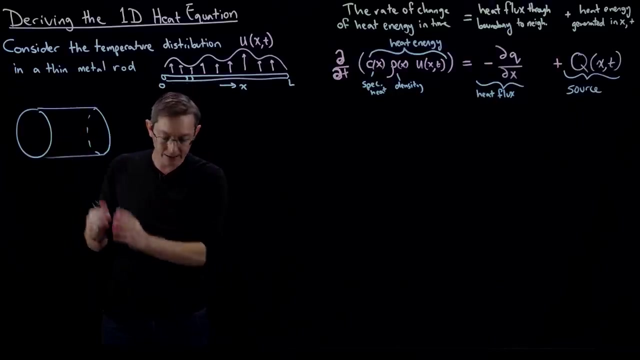 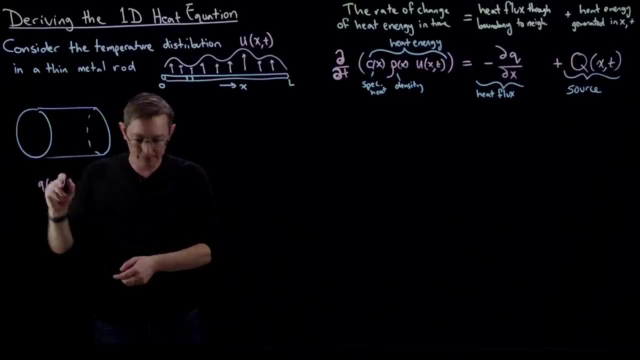 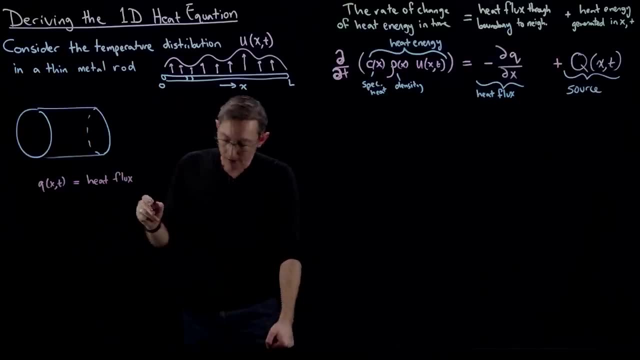 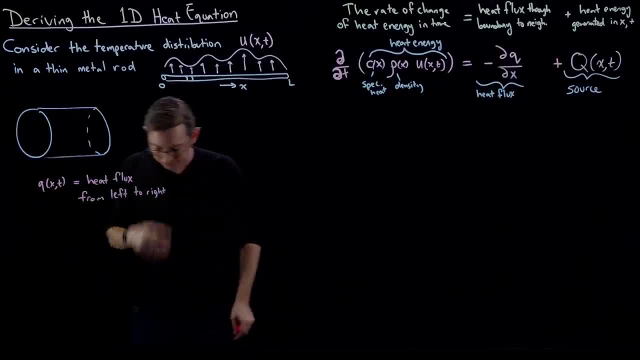 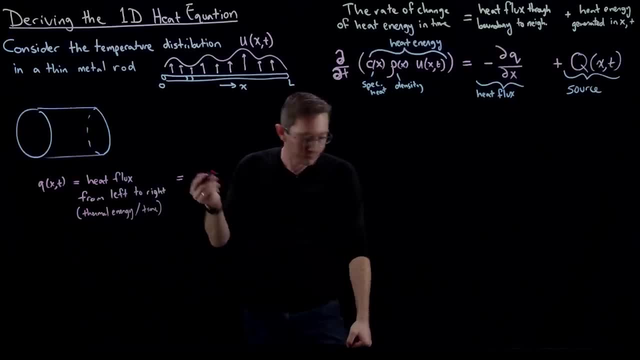 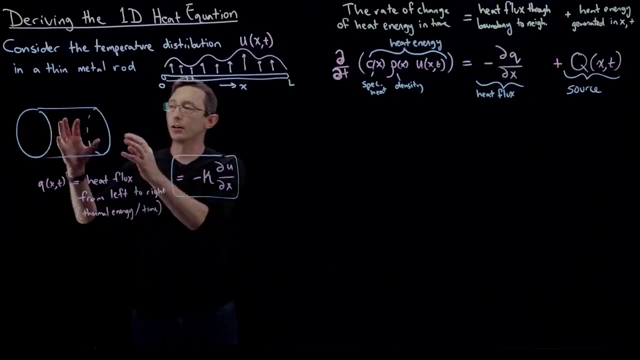 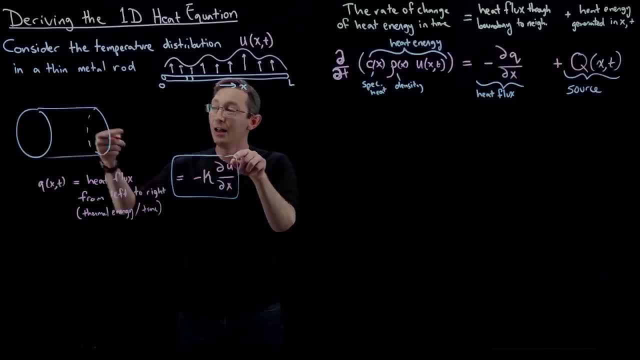 temperature in space, that this is partial u, partial x, meaning there is a change of temperature in the x direction. if i have that partial u, partial x, then i expect there to be a large heat flux at that location. okay, so the heat flux at a location x is directly proportional to the gradient. 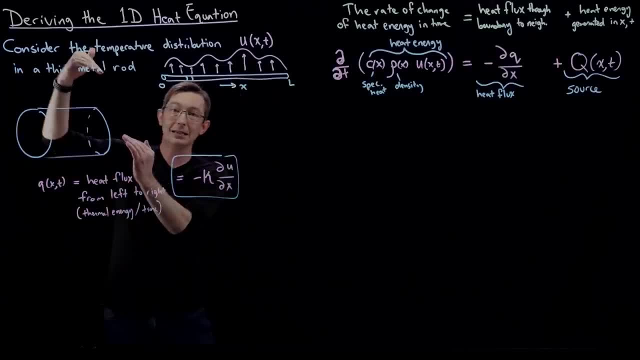 of the temperature at that point x. so if i have a really steep temperature gradient, really really hot on one side, really really cold on the other, this is a big number and i get a lot of heat flux. this is common sense, okay, but it was. you know, this took a long time to be derived. 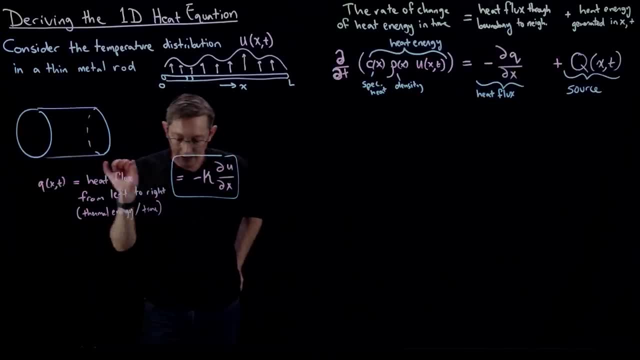 this is a major result. so this q of x and t? um, what i want to do is actually like write this down, so we have q kind of coming in here. this is q? um at x and t, q of x and t, and there's also some 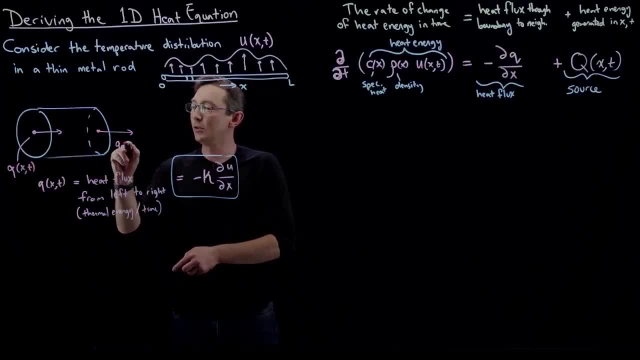 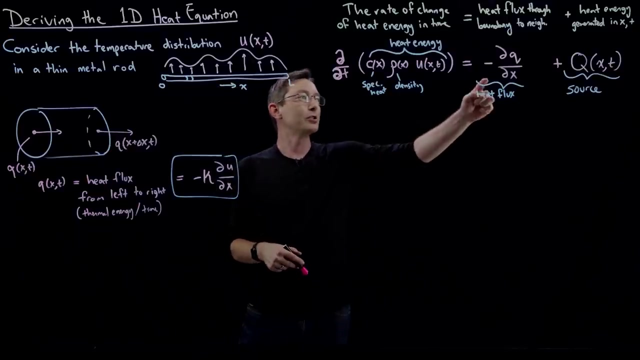 little infinitesimal heat flux out. this is q at x plus delta, x and time, and so if these two are equal to each other, if the, if the, if the amount of heat flux in is equal to the heat flux out, then this term is zero. there's no rate of change of heat energy in this little volume, and so that kind of tells you why. 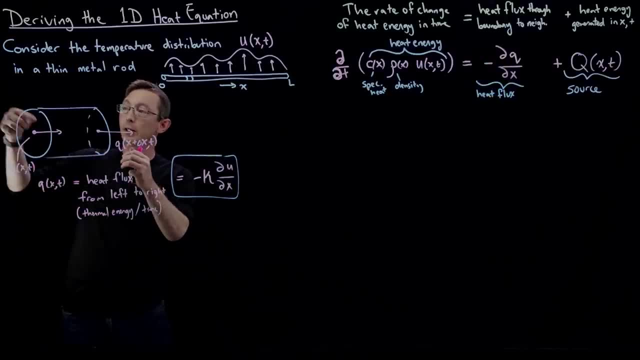 now, if there is a gradient in this heat flux, if i have more heat flux coming in than going out, then this is discharging out the heat flux and the heat flux is going to be discharging out the heat. This should be a net positive rate of change of heat energy in this volume. 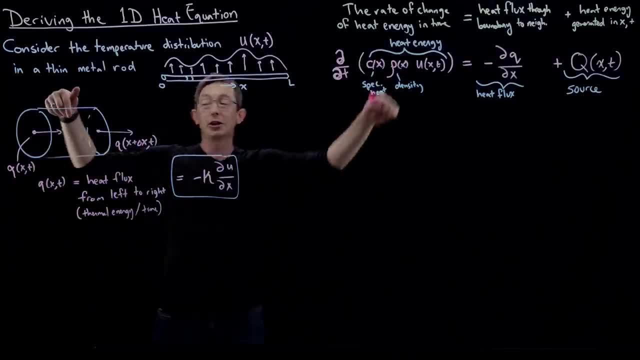 If I have more heat flux leaving than entering, I should have a net rate of change decrease in the total heat energy in this volume, And so it's always a pain for me to get this sign right. but basically what we are computing is this: partial Q, partial X. 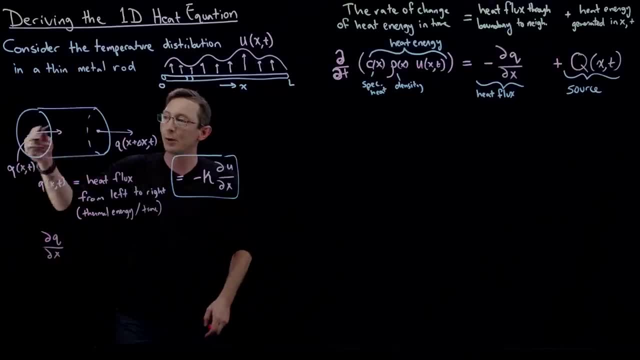 The gradient of this Q heat flux tells me roughly if heat is, on average, entering or leaving this little infinitesimal volume. And so this is like the limit, as delta X goes to zero of Q of X and T, minus Q of X, plus delta X and T divided by delta X, and that's minus. 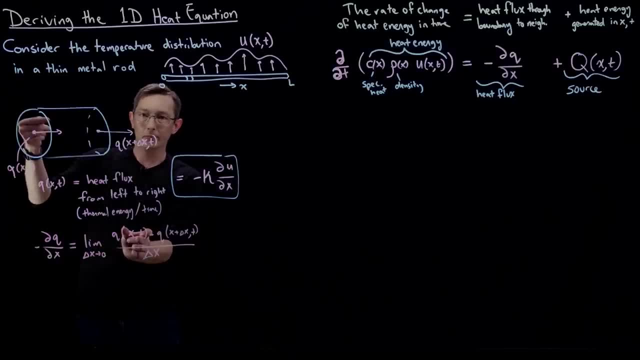 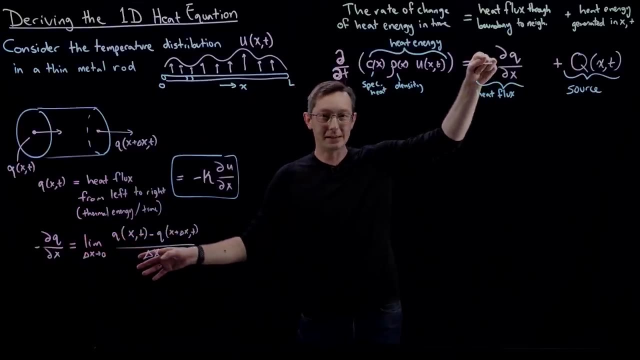 So essentially what this says is that if I have more Q coming in, then I have more Q leaving, then I have this kind of. I always get the signs mixed up. let me try to do this really, really carefully. What I'm trying to do is I'm trying to figure out why this is a minus sign and try to convince. 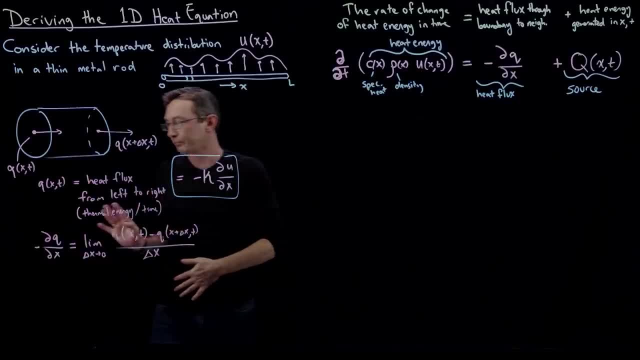 myself that this is actually correct. So let me just slow down a minute. If I have a negative gradient of Q, what that means is that Q is bigger coming in than going out. Q is bigger than medium, than small. That is a negative gradient of Q. That is a negative partial Q. partial X. 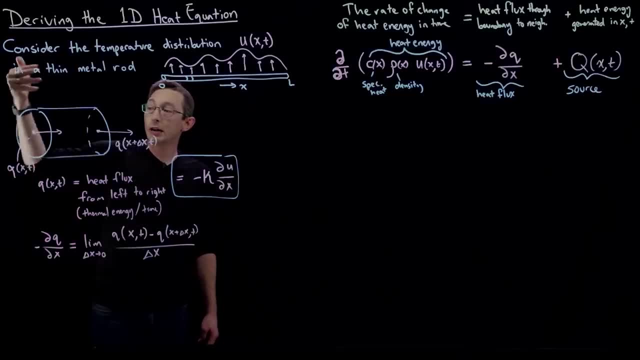 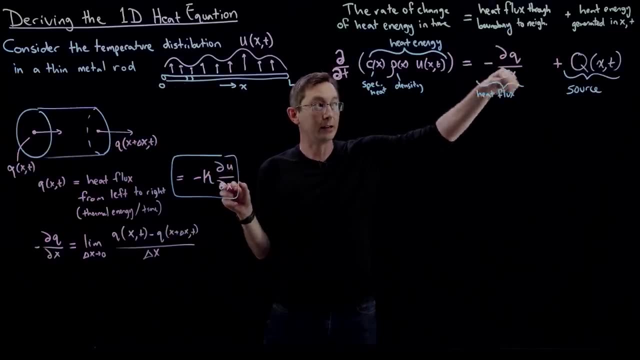 And if I have a negative gradient of Q, that means I have more heat energy. this one's bigger than this one. I have more heat energy entering than leaving. So if I have a negative gradient of Q with respect to X, I have a positive rate of change. 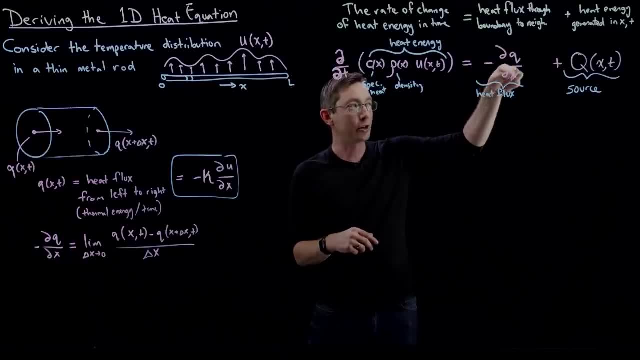 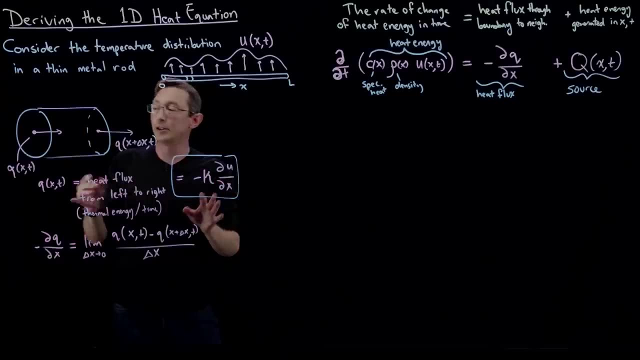 of heat energy in that little volume. So when Q- partial X is negative, this should be positive and that's why I have that little negative sign out there. So this does fit with the convention that if I have a negative gradient of heat flux, 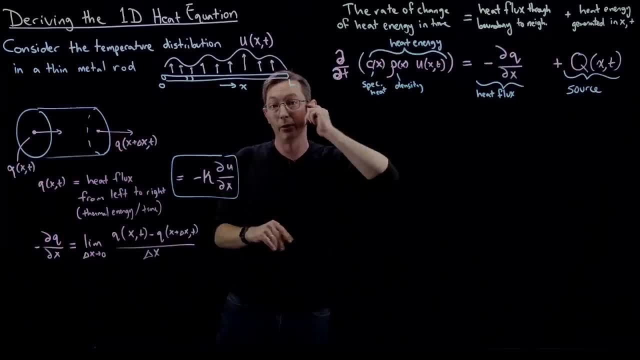 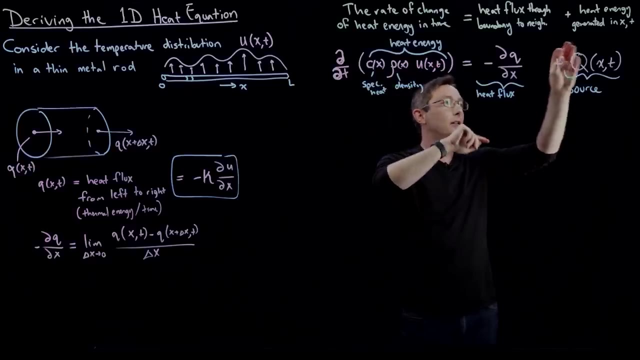 Q that should have an increase in the heat energy in that little point X. Now this Fourier law of heat conduction is really important. That's how we right now. what we have is a partial differential equation in terms of Q and Q and little q. 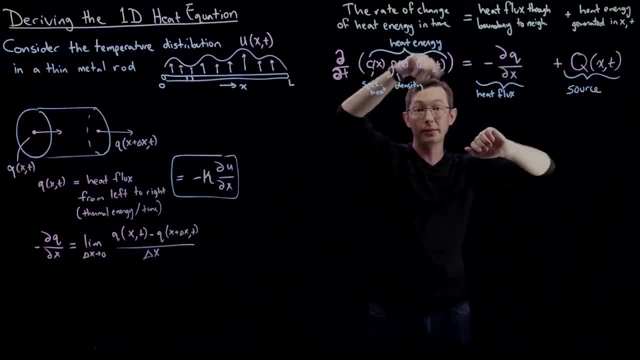 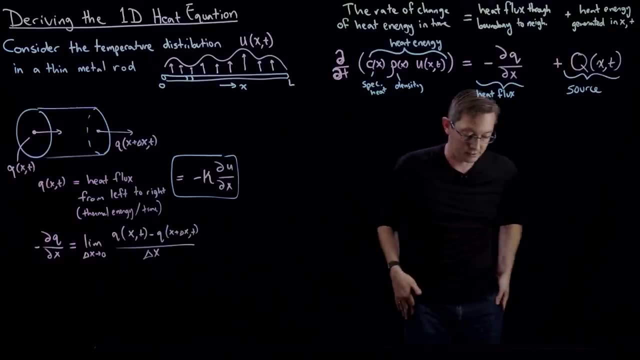 And what I want is to write this all as a little partial differential equation of U, the temperature. So I want to relate my heat flux directly to the temperature, And that's what the Fourier law of heat conduction allows us to do. So maybe I'll just give you a tiny little aside. 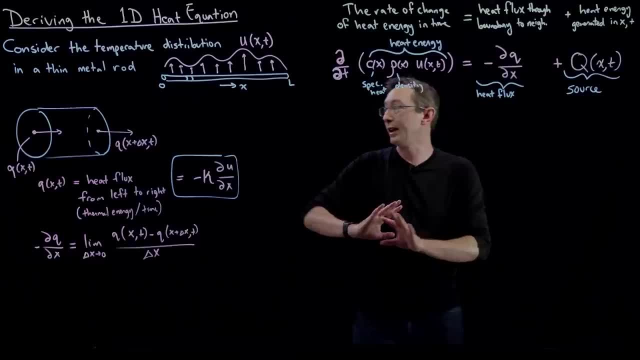 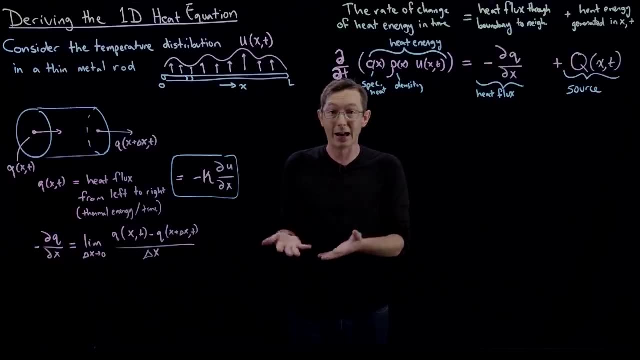 This is where Fourier enters, and this is not for the last time. So Fourier has a treatise on heat conduction. It's a beautiful book- You can still read it today, translated- and it actually gives his thought process As he is deriving these equations and analyzing these equations. it's quite interesting. 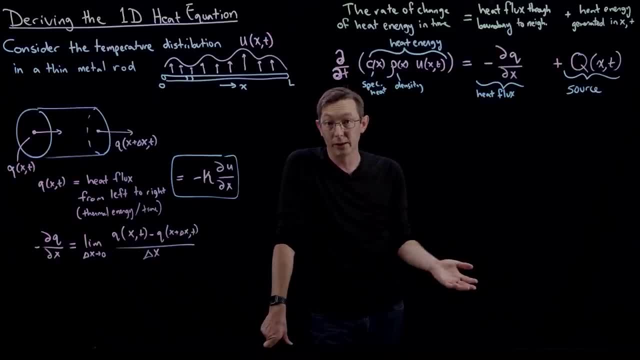 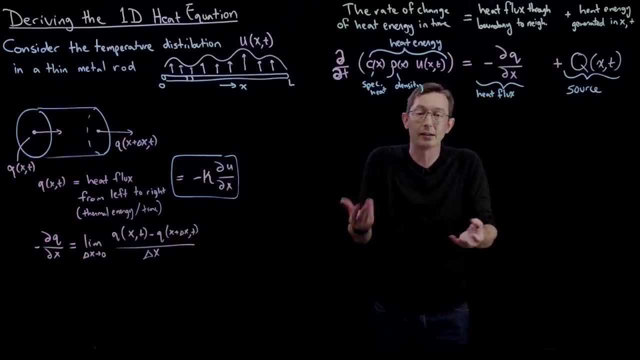 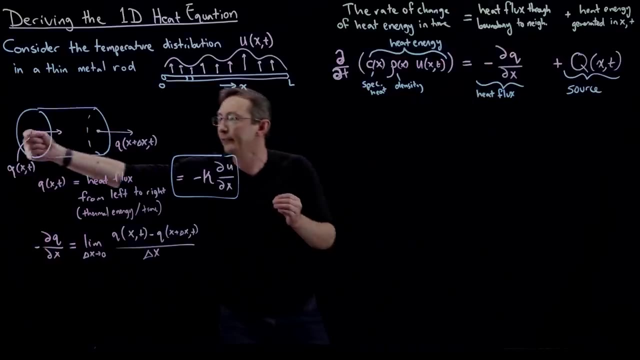 And actually the heat equation is why Fourier developed the Fourier transform in the first place. So we'll see that later. And so Fourier made these three observations. He did experiments or he collected the information from other people's experiments- Newton's experiments and others' experiments- that there is no heat flux when the temperature 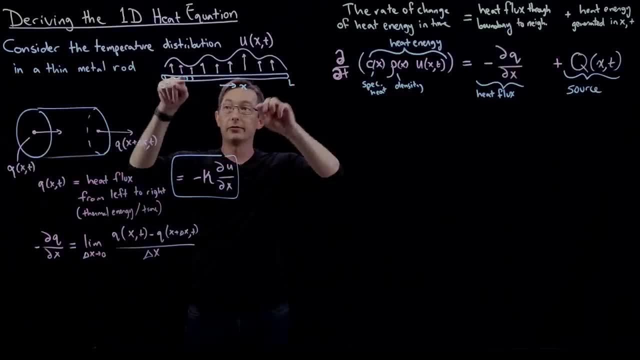 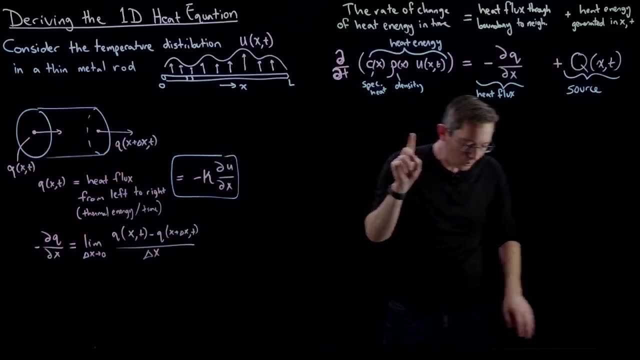 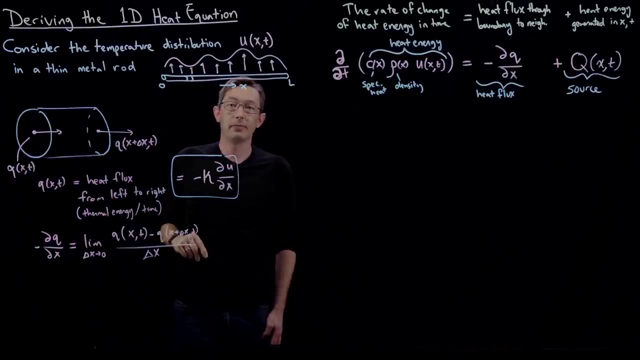 is constant. So if the temperature in this rod is constant, from you know, at a point X- if it's the same temperature to the left and to the right, there will be no heat flux. That's the first observation. The second observation is that heat energy flows from high temperature to low temperatures. 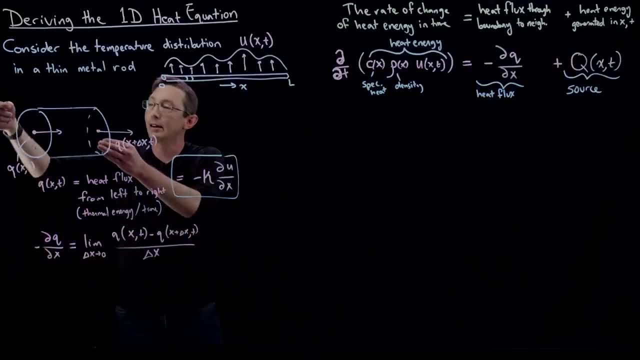 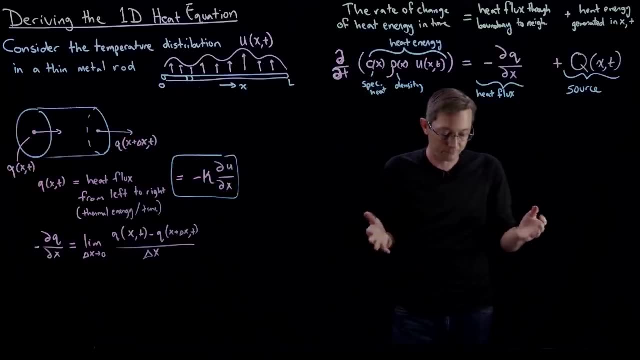 So if I have a high temperature on the left and a low temperature on the right, I will get a net flux of heat energy into this low temperature region. So heat flows from high temperature to low temperature. That's also observed. That's the second property. 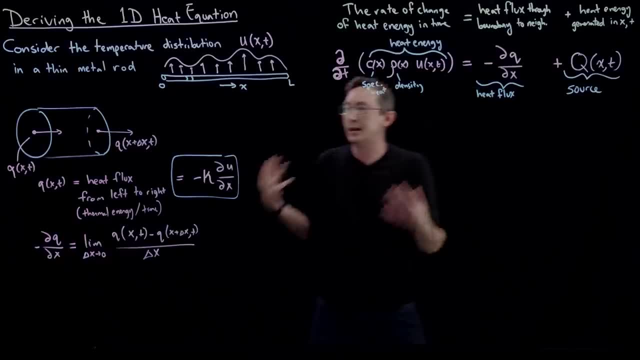 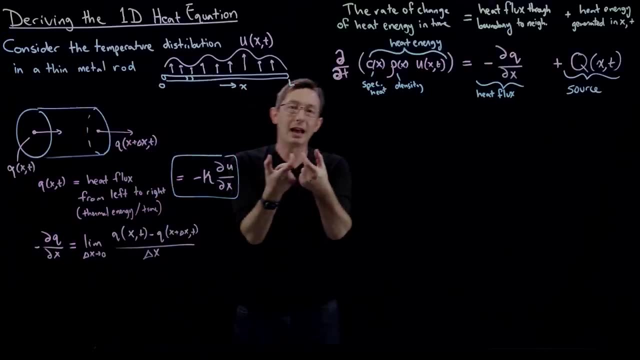 And the third property is that there is more heat flux. The third property is that there is more heat flux when there is a larger temperature difference. If I butt up two little pieces of metal and they are 10 degrees different, that will change. 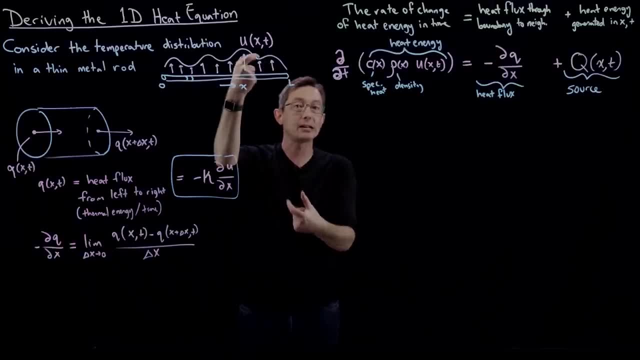 conduct heat less fast than if there's 100 degrees difference. The bigger the temperature difference, the faster the heat flux, And so, essentially, if you put all three of those together, you get Fourier's law of heat conduction, which is this expression here: 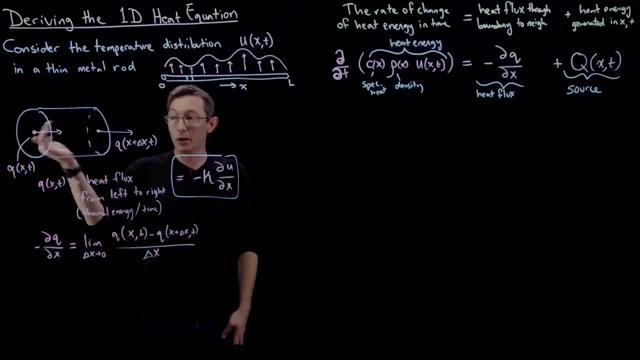 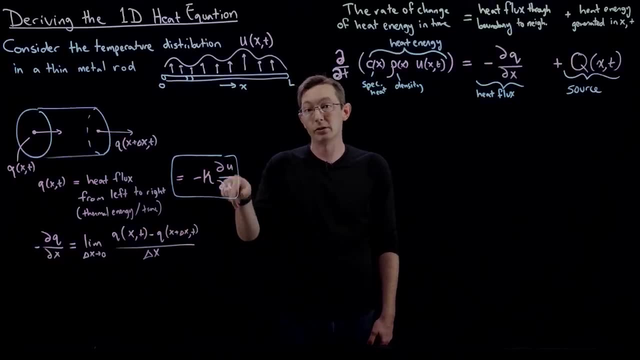 The heat flux from left to right, the thermal energy flow in time. The heat flux from left to right is equal to this, minus kappa, times partial u over partial x. the gradient of u with respect to space. the derivative of u in space. 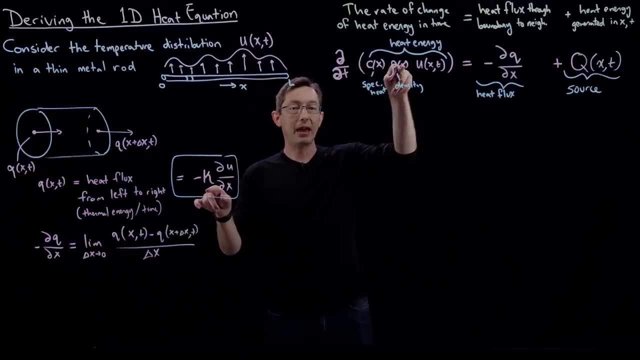 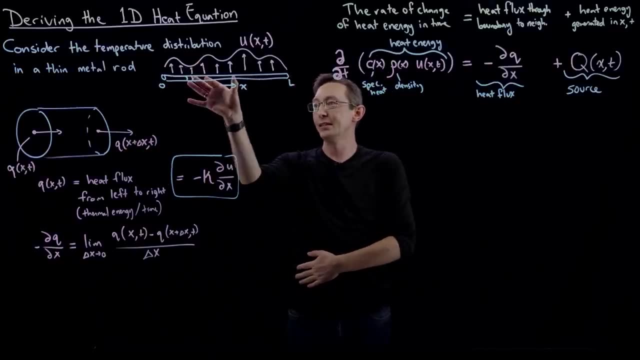 This kappa is really a kappa of x, Just like my specific heat and my density. I explicitly made these functions of x because I might have a weird material where it's copper here and then it's lead and then it's a mixture of copper and lead. 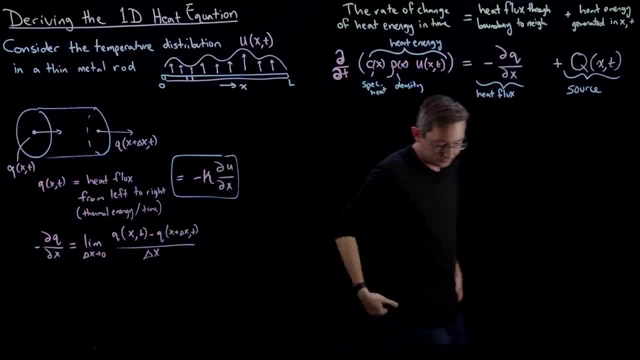 These properties can change in space. Okay, good, And so that's the third property. The fourth property is that there is more heat flux than there is in time, And so if I butt up two little pieces of metal and then there's 100 degrees difference, that's. 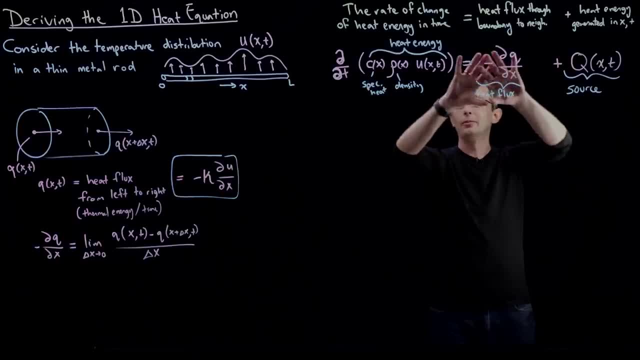 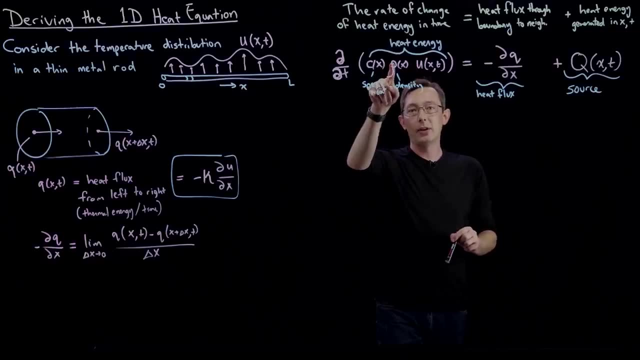 the third property, And so this Fourier's law of heat conduction allows us now to write this PDE in the following way, And you'll notice that c and rho are not functions of time, so I can pull this partial derivative. so it's hitting u. 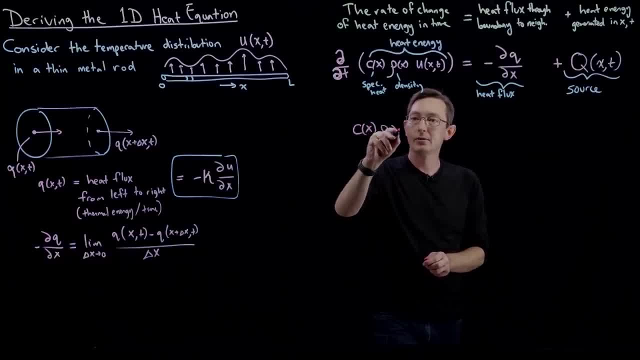 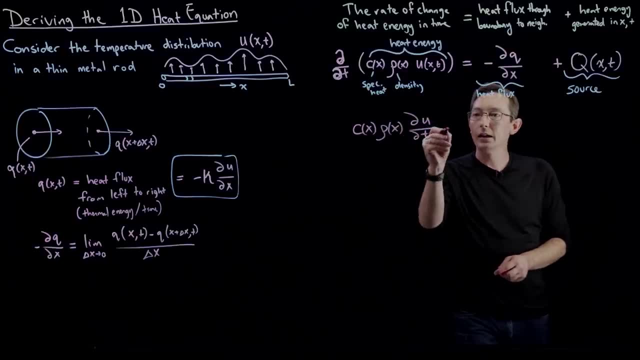 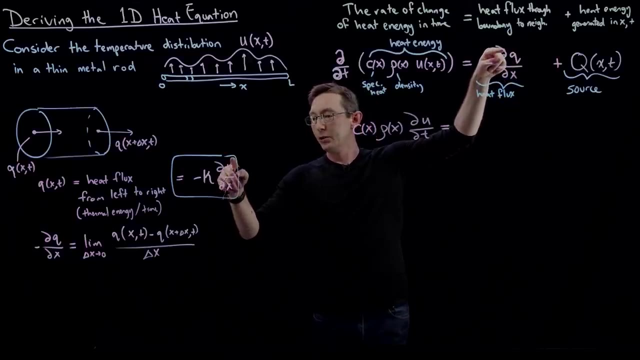 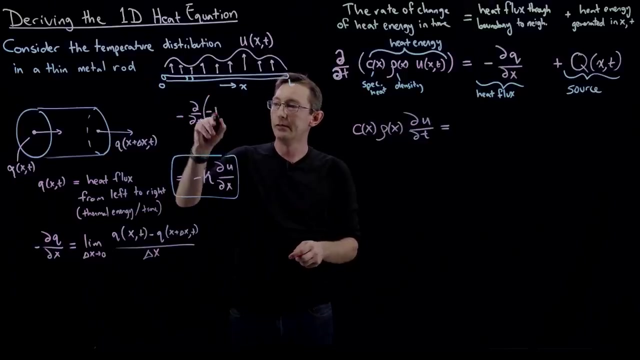 And so what I have is I have c of x times rho of x times partial u, partial t equalsnow I have a little q of partial x, the partial of q with respect to x. Because q is partial u, partial x. maybe I'll just write this out: negative, ddx of negative. 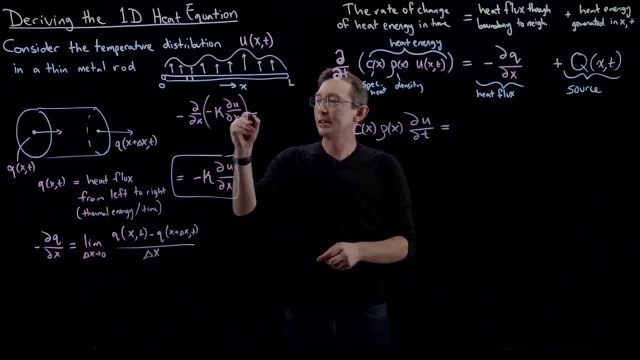 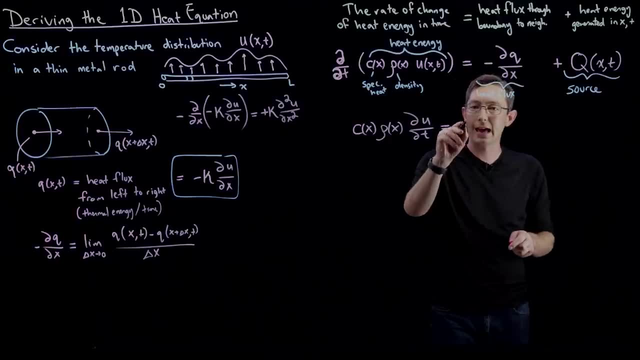 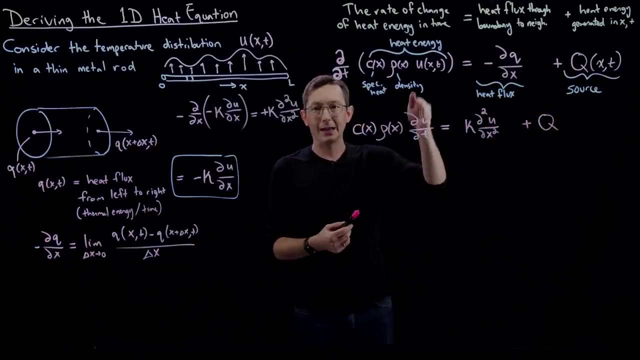 kappa partial u partial x is just positive. kappa partial squared, u partial x squared. So this equals kappa partial squared u partial x squared. Good, Plus my source term And I've dropped u as a function of x and t, big Q as a function of x and t. 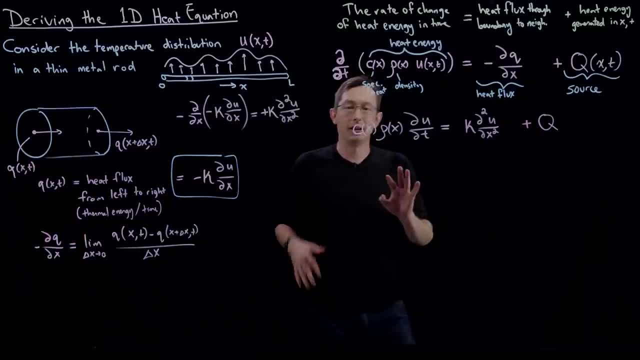 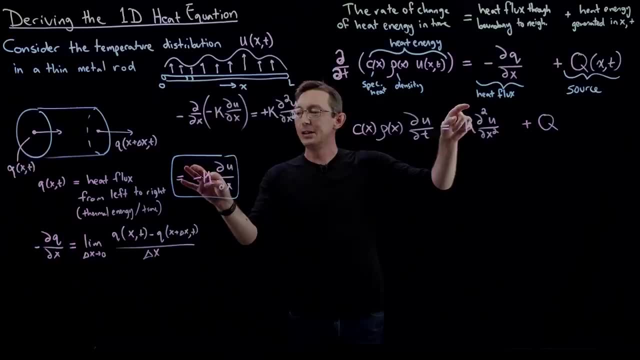 I have actually, you'll notice here I cheated for expediency's sake. I am assuming that this kappa is a constant. this kind of this is the rate of thermal conduction, kind of how much heat is conducted, the conductivity. 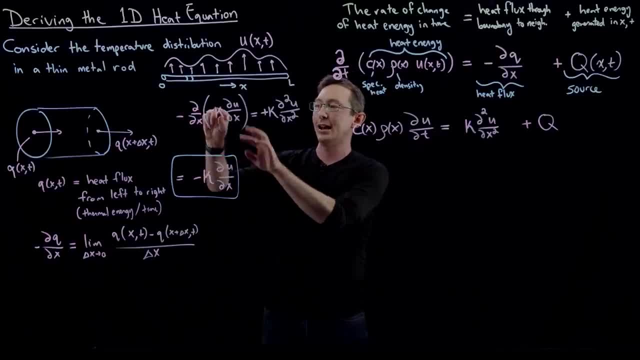 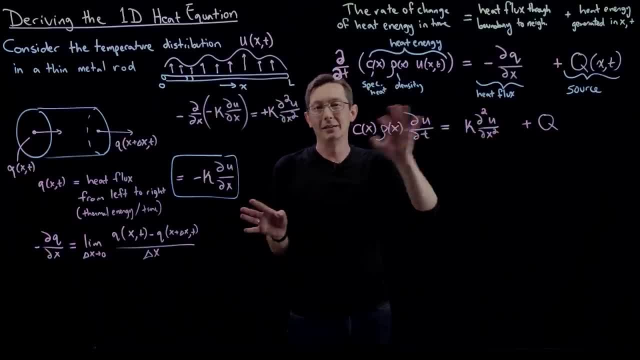 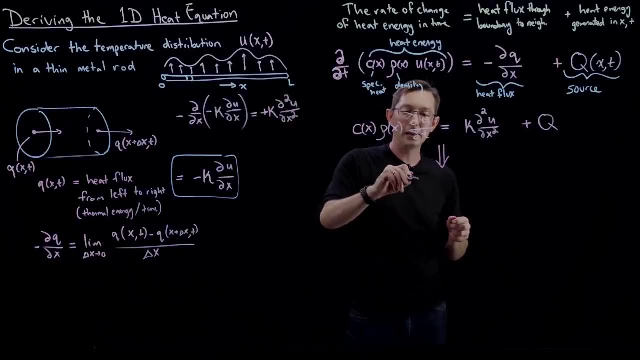 more complicated expression here And so I've kind of simplified my life. And if you simplify and basically say that you know c? rho and kappa are constant in space, then you get this nice expression that partial u, partial t equals kappa over c? rho. 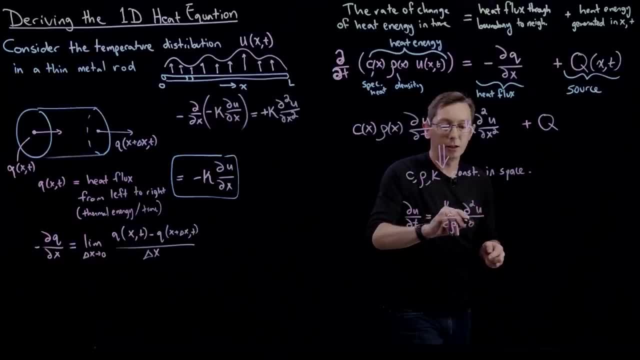 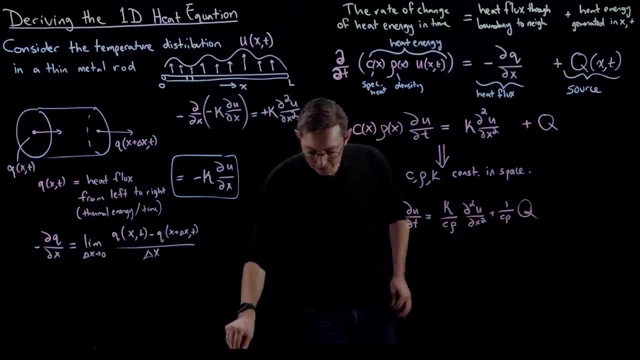 partial u, partial t. Partial squared u, partial x squared. plus this constant, you know, 1 over c rho times my forcing function, And that is essentially. I'm going to box this. I think we did it. This is the heat equation. 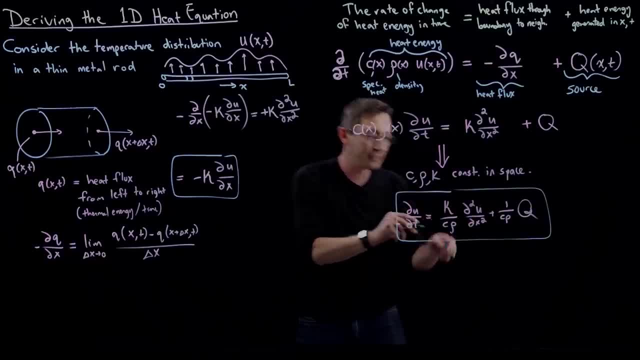 This is the diffusion part of the heat equation. This is the diffusion constant, This is that positive constant, alpha squared we talked about before. that, just you know, tells me how heat is diffusing And this is any forcing term. You know, if I hit this thing with a blow torch. if there are atomic, you know fission. 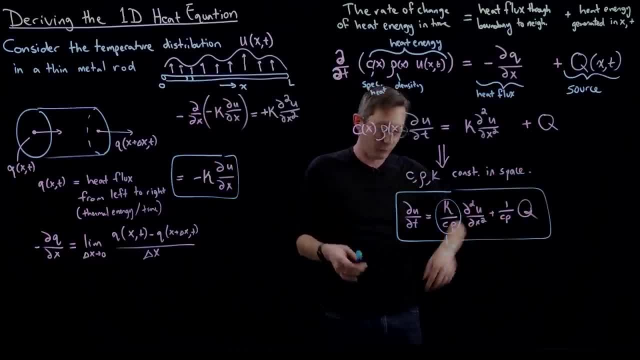 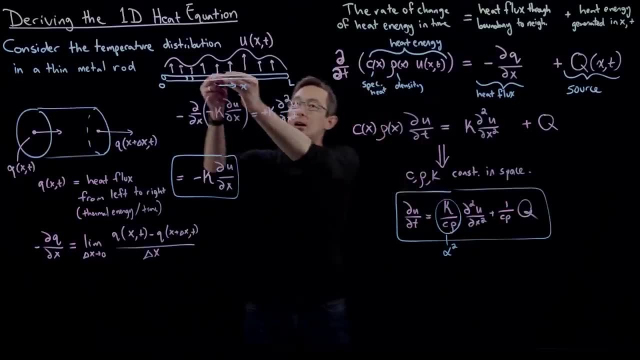 processes causing heat energy to create. this is the forcing term here, And so this is pretty cool. This is the actual full-on heat equation for a constant material: 1-D thin metal rod. Okay, good, So in future lectures, what I'm going to do is I'm going to generalize this for 2-D, 3-D. 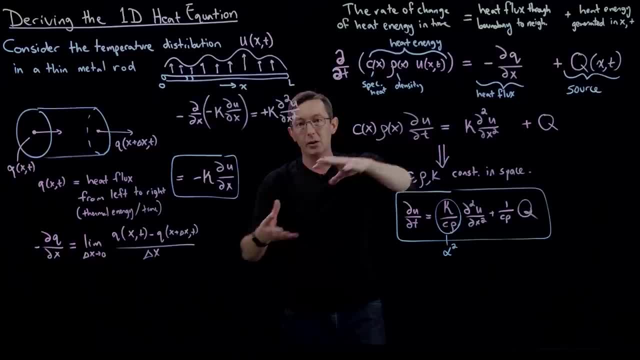 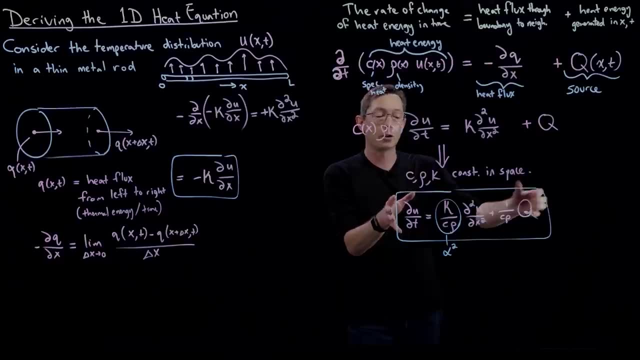 N-D. We're going to derive the n-dimensional heat equation, for you know a, you know a, you know a three-dimensional object like the Earth, or something like that, And it will be a partial differential equation where now this will be the Laplacian of U. 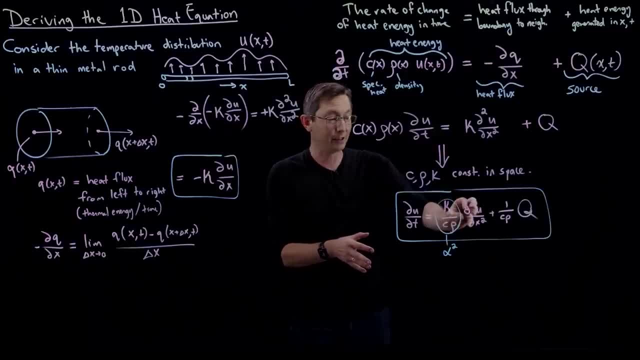 Okay, instead of just a second derivative with respect to X, it'll be the Laplacian of U. In fact, I'll just write down, you know, we'll essentially get U sub T equals alpha squared Laplacian of U. in the absence of forcing terms. 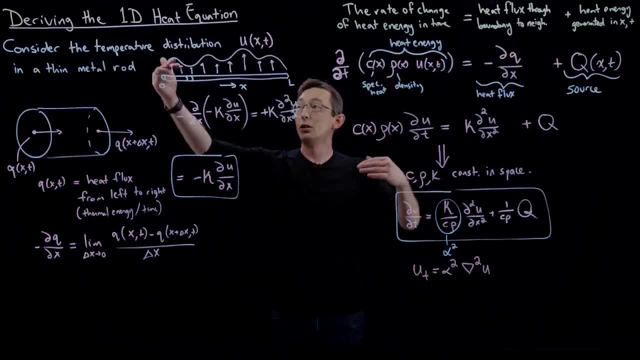 So that's one thing we'll do. We will also look at how do you actually solve for Laplacian. We will solve for the heat distribution, given you know initial conditions and boundary conditions and source terms. We will solve for the steady state heat equation. 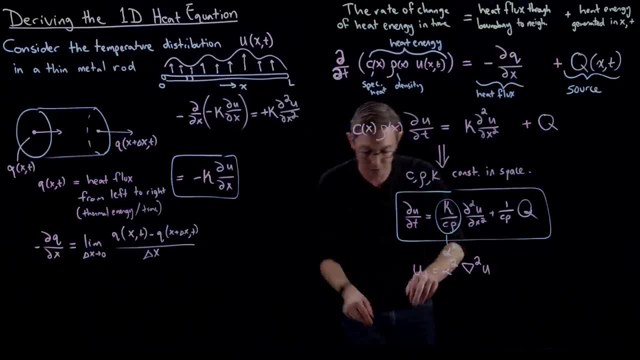 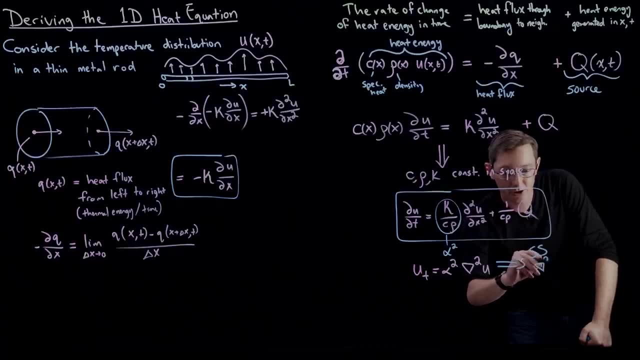 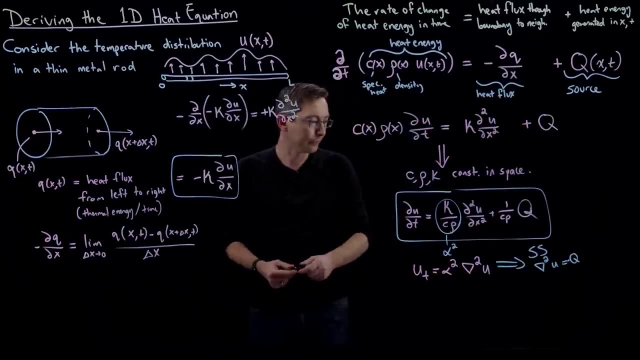 So if in steady state, this partial U, partial T is zero, this partial U, partial T is zero, And so in steady state, in steady state we have the Laplacian of U equals zero. Or if there's forcing minus Q, Okay.